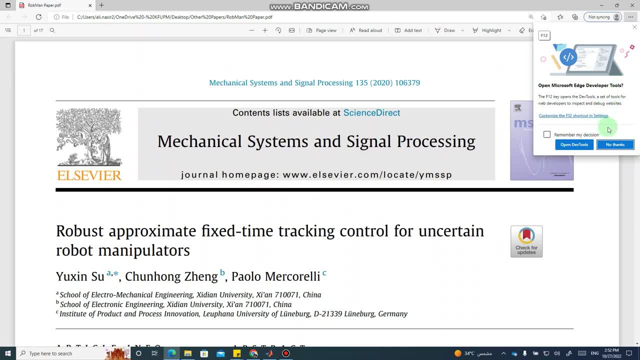 Bismillahirrahmanirrahim, Assalamualaikum, dear students, Welcome to the online lecture on MATLAB simulation of control systems. Today we are going to discuss this new paper: Robust Approximate Fixed Time Tracking Control for Uncertain Robotic Manipulators. 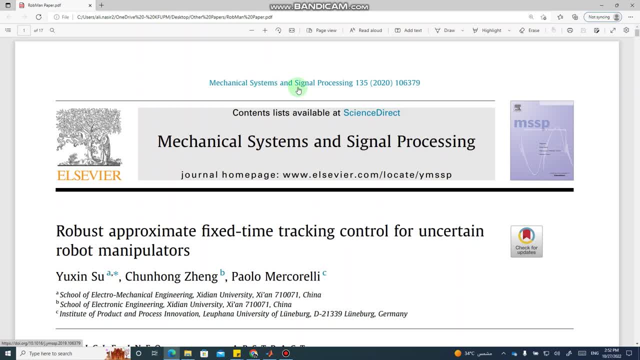 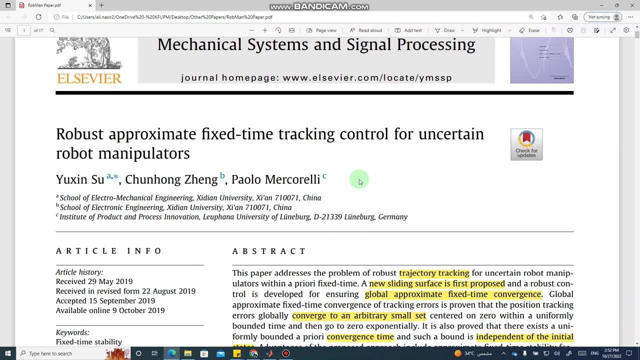 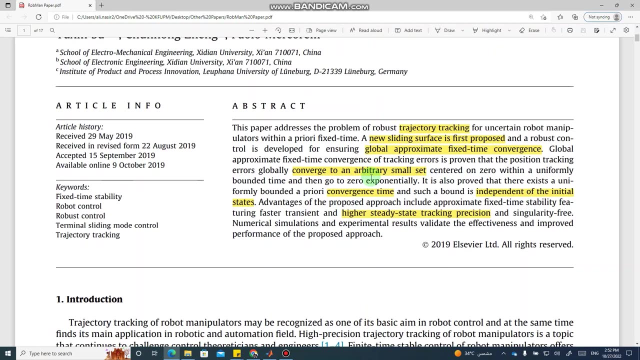 This paper has been published in Mechanical Systems and Signal Processing in 2020 and it's fairly recent and has been shared by one of the viewers of the channel, So I am thankful for the reviewers who share latest and useful papers. Please note that I cannot simulate all of the papers that you share with me, because of different reasons. 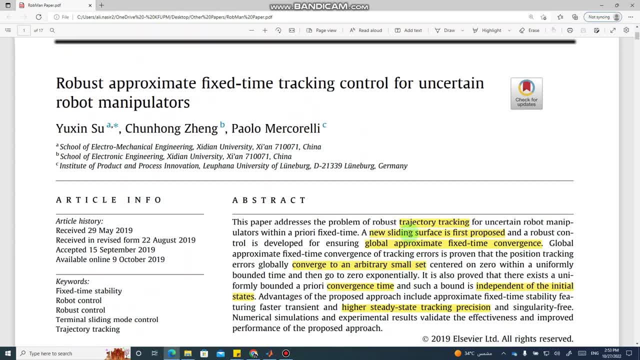 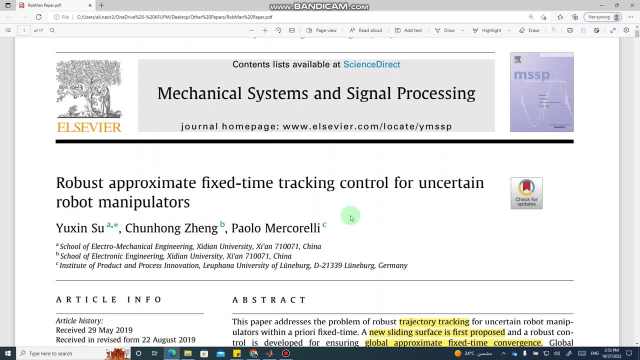 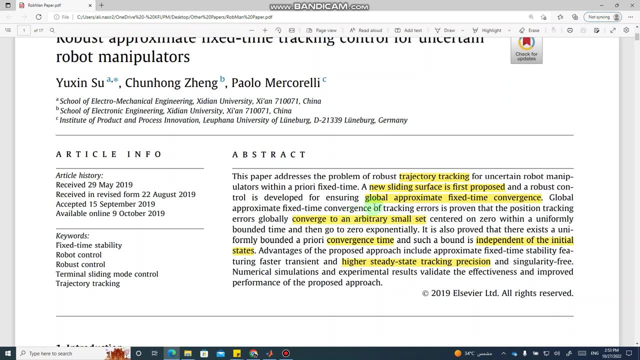 Mostly, you have to understand that there are a lot of problems. There are a lot of papers which do not provide enough information within the paper itself that is required in order to simulate the results of the paper. But many of the good papers do provide this information. 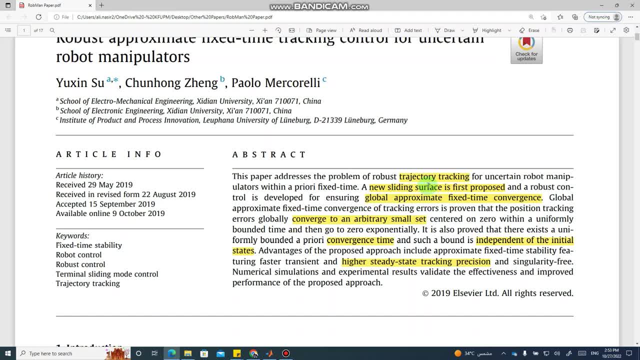 So here I will try to make this channel focused towards latest and more impactful research. There have been a lot of requests regarding the model, predictive control and reinforcement learning. I will look into these as I find time from my schedule. So stay tuned with the channel. So hopefully, you know, in the long term, 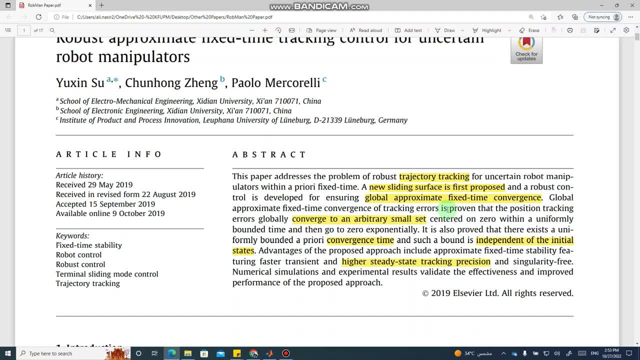 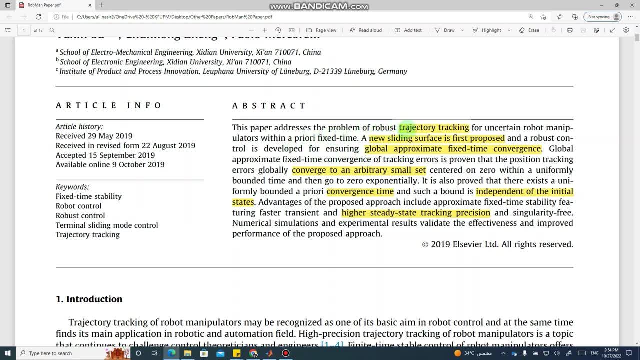 will have papers that are important and they're that are impactful in the control systems engineering research. This paper addresses the problem of robust trajectory tracking and a new sliding surface is first proposed, and this controller provides global approximate fixed time convergence and convergence to an arbitrarily small set, which is centered. 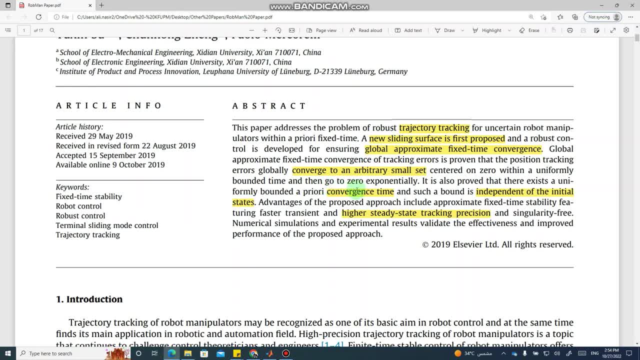 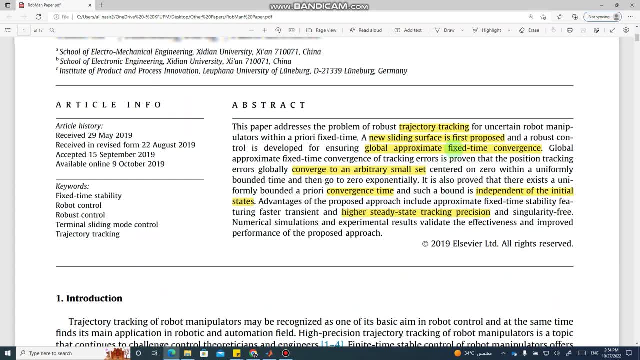 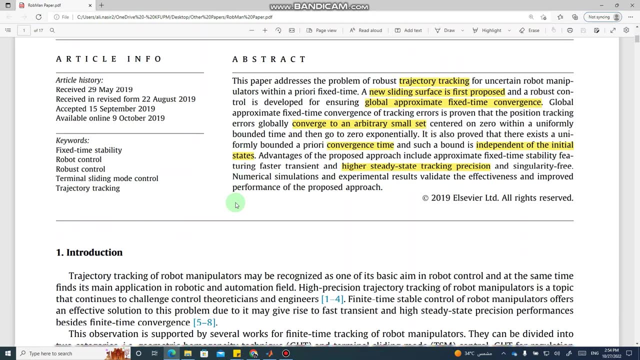 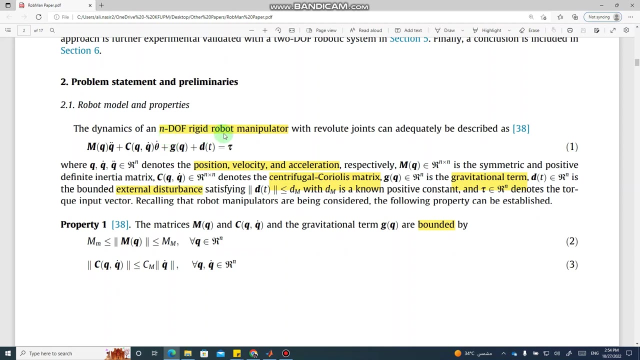 around zero within a uniformly bounded time. so overall it's a. it looks a very useful and good controller for, at least for the uncertain robot manipulators. and as always, we will not go into the much details of the paper, we will just look into the system. so this is the n degree of freedom: rigid robot manipulator. 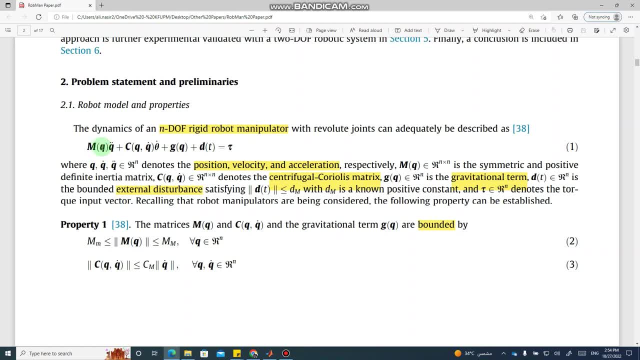 dynamics. you can see here. this is the, the matrix, the dynamics matrix and the centrifugal choreography, this matrix C and gravitational term G. so these are. this is pretty standard model and in the end they have given the example of two degree of freedom, robot mode manipulator. so we will be simulating a two degree of freedom there. 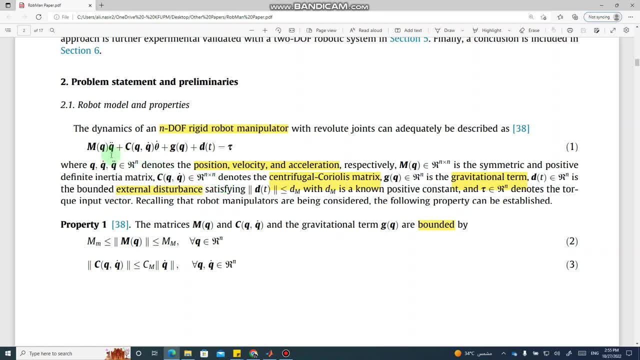 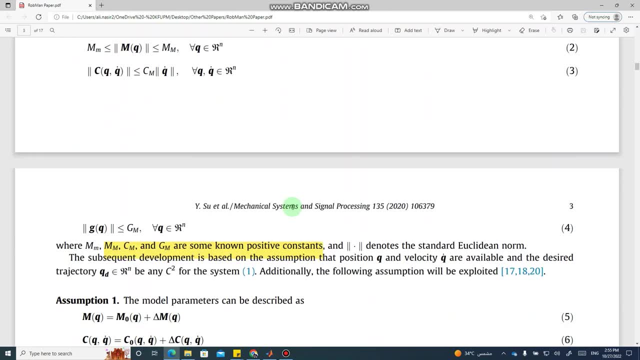 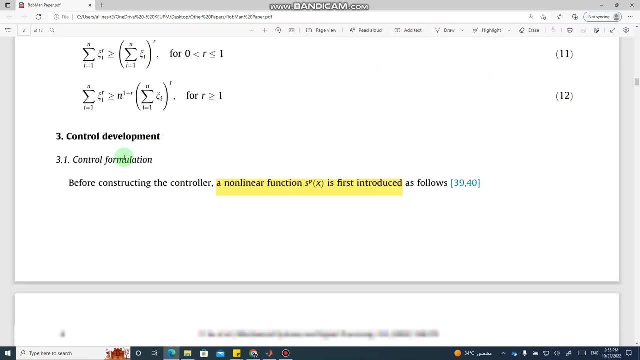 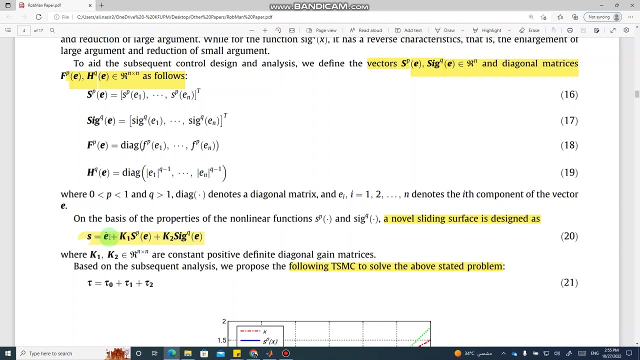 and in will be equal to two, and this Q are the angles and angular rates of the robotic joints. so the control that has been proposed in this paper is basically basically this one. so this is the sliding surface that has been proposed in the paper. S is equal to the derivative of the error plus k1 times. this is a special signal. 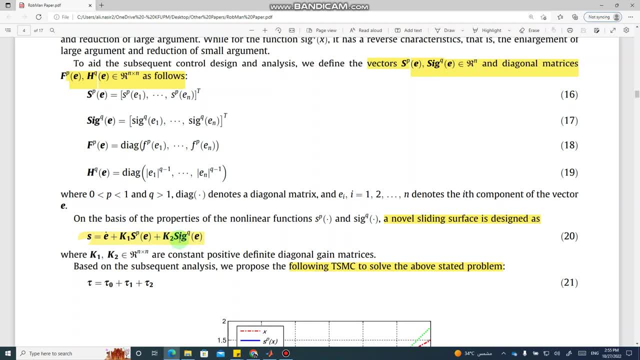 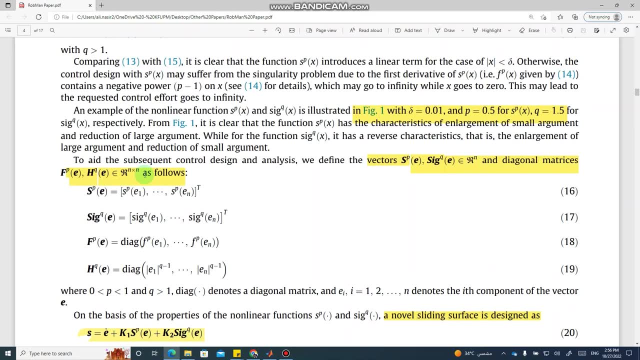 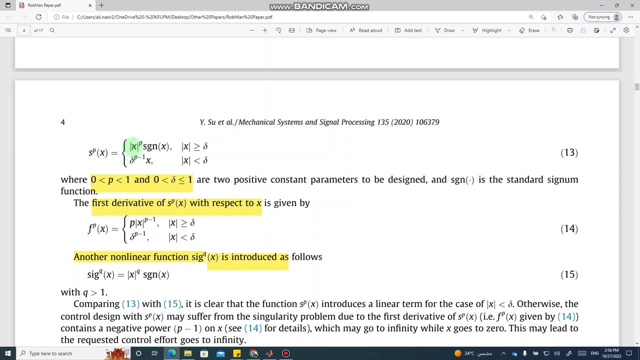 function SP of error, and k two times another special function, privacy power Q of error. so sig power q. this function has been defined here. so this is sp function. sp of x is equal to magnitude of x raised to the power p into sine of x, where x is greater than equal to some number. 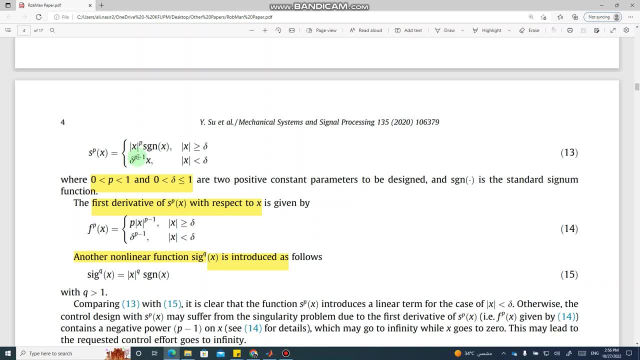 delta and sp is equal to delta power, p to the power minus 1 times x when x magnitude is less than delta. and similarly, this is fp function, which is equal to f, p into magnitude of x raised power, p minus 1 whenever magnitude of x is greater than equal to delta, and it is equal to delta raised. 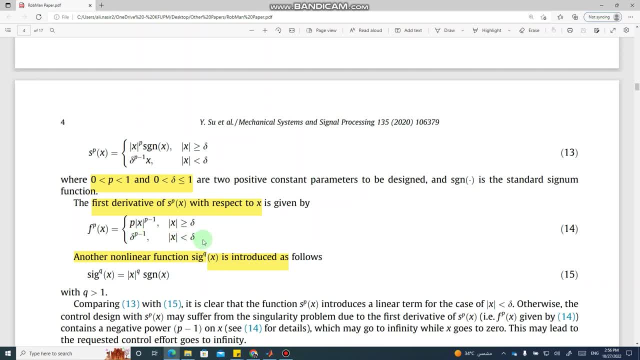 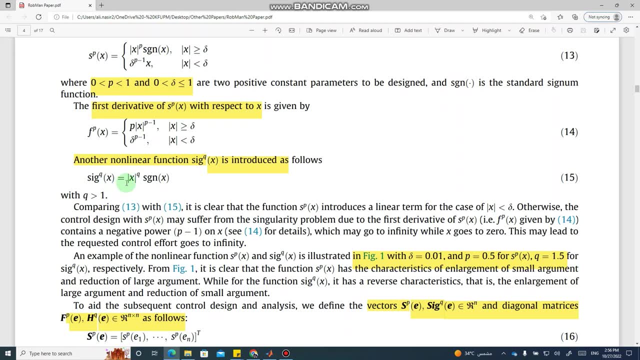 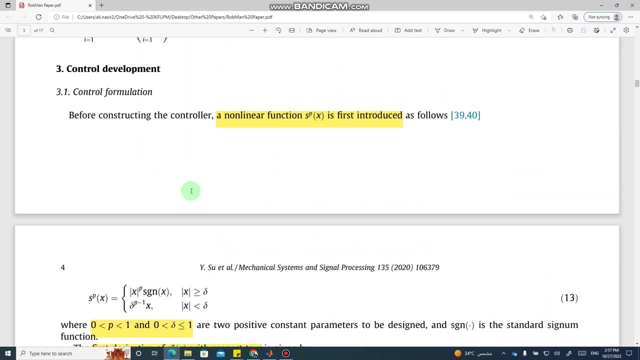 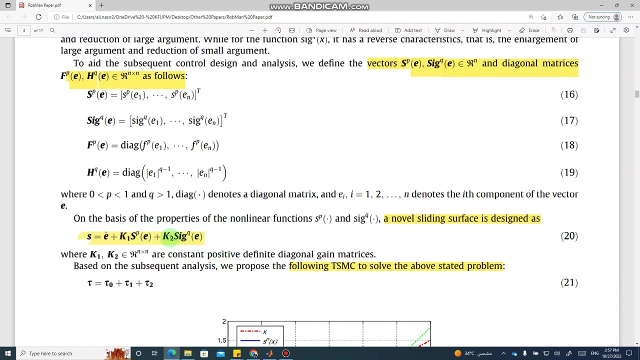 power p minus 1 whenever x magnitude is less than delta. so and, and this sig q x function is just magnitude of x raised to the power q times the sine of x. so they have defined these functions for making these equations look less messy. so this this is. you know, you can see this equation written in a nicer way because these two 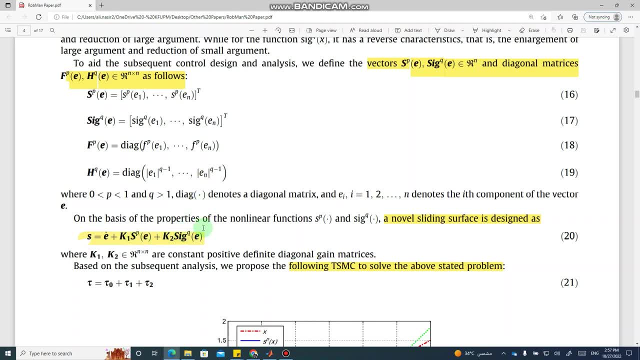 functions sp and cq have been defined above for a vector case. this is just component wise function. sp you take for each component, then that will be the sp of a vector. similarly, sig q of e a vector is a sig q of each of the components. similarly, fp of a vector is fp of each of the. 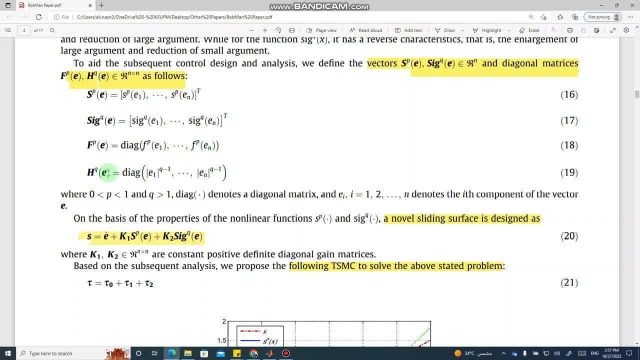 components. hq is not defined separately. it's just defined right here that hq of a vector is a diagonal matrix where each of the diagonal entry is magnitude of a component of the vector raised to the power q minus 1. we will be using these in our control simulation today, so 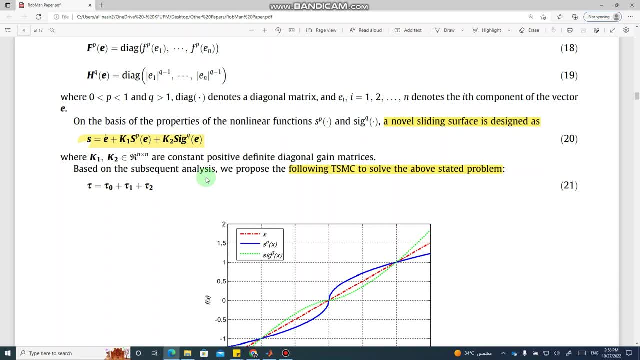 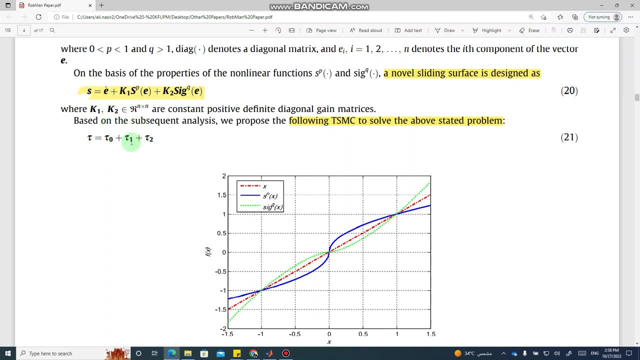 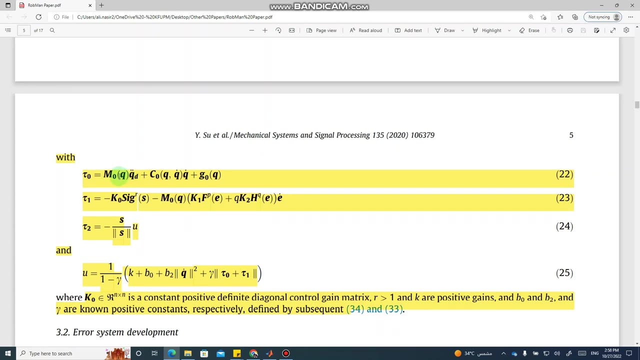 if you just one second, okay. so the total control is: tau is equal to tau naught plus tau 1 plus tau 2, they have it has three terms- and tau 0. this has been defined here. so here m 0 and c 0 are and g 0 are matrices with nominal values of the mass and radius etc. but 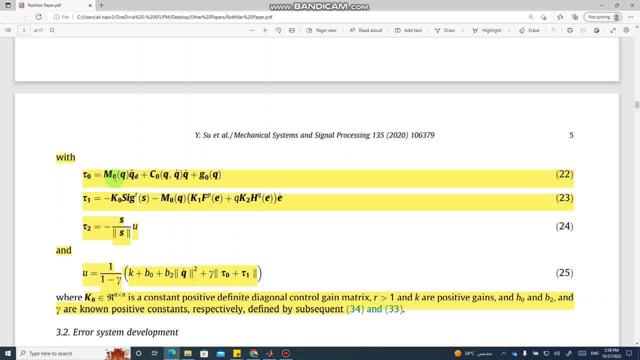 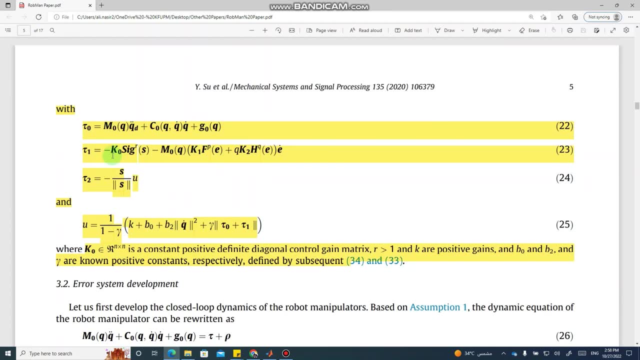 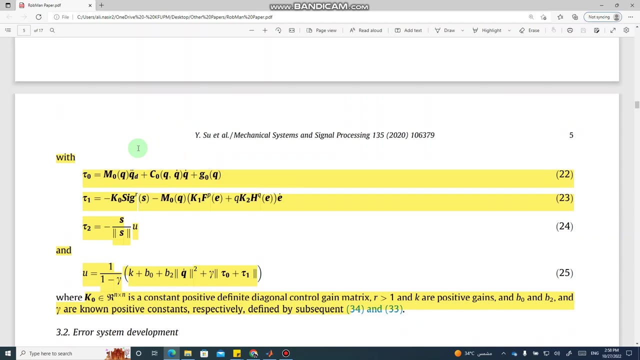 you can use the actual value if you know the actual value, and you can use the nominal value if you don't know the actual value. when you, if you only know the nominal values, then tau 1 is: is this: sig power r is same as sig power q instead of q we have r here. so there, instead of q, here we. 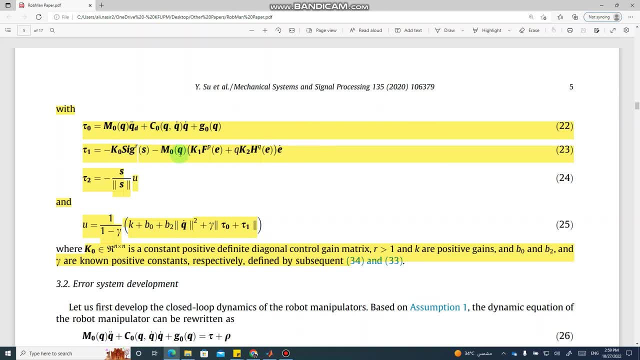 have r and m m naught times q, so times k1, fp. fp is the function fp that we saw above, so it's the fp function of error and then hq function of error. we also saw this above, and tau 2 is minus s over. 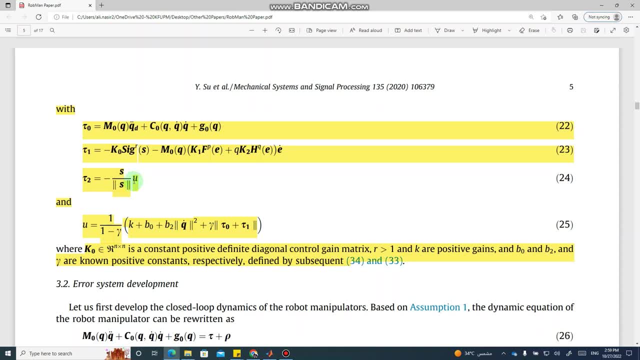 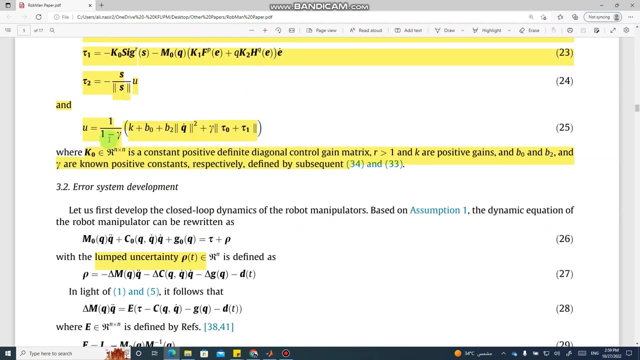 magnitude of the norm of s, the sliding surface times u, where u is 1 over 1, minus gamma times k plus b, naught plus b2, and so so this is the total control law that has been developed in this paper. similarly, this gamma in the, in this sub sub term of the control u. this is some. 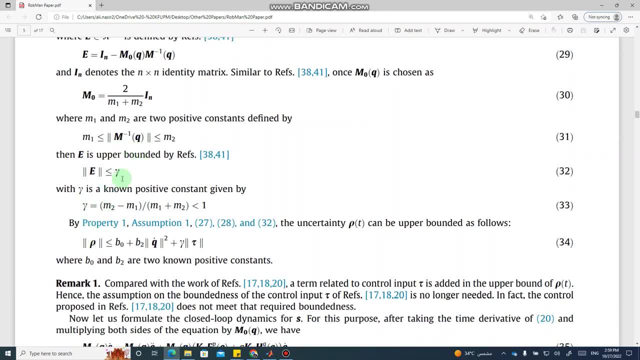 uh, bounding term between 0 and 1. so this gamma is given by. you know this. this, this is nominal matrix. if you bound the norm of the nominal nominal matrix by m1 and m2 from above and below, then gamma will be m2 minus m1 divided by m1 plus m2. 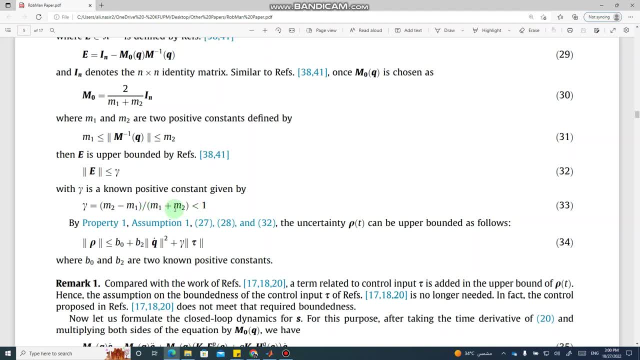 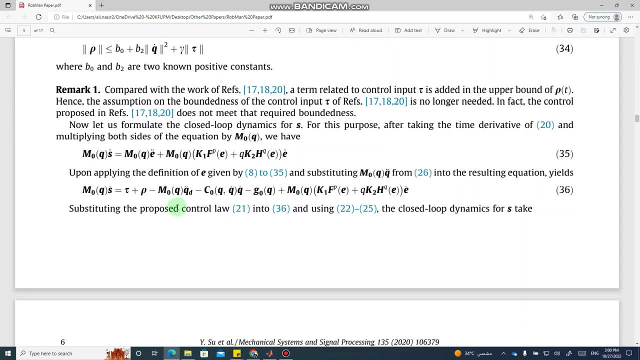 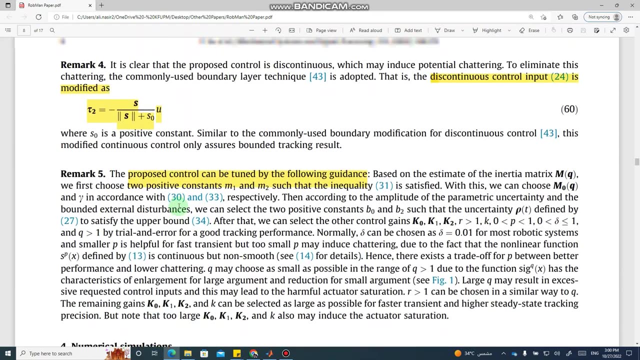 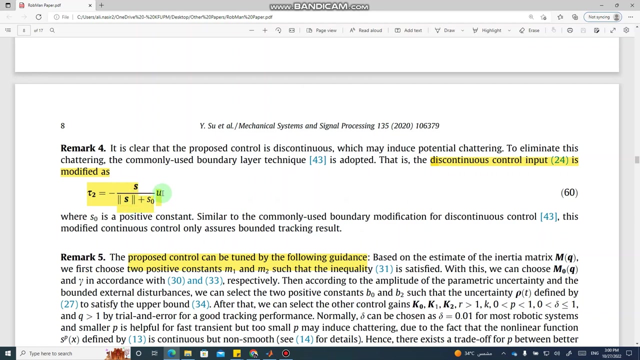 less than 1. so it's. it's basically a number between 0 and 1. so, um, here, uh this, let's go right to the end. so here there's another remark: that instead of tau 2 being s over norm of s times u, you can also have tau 2 to become s over s norm, plus s naught into u. that will make 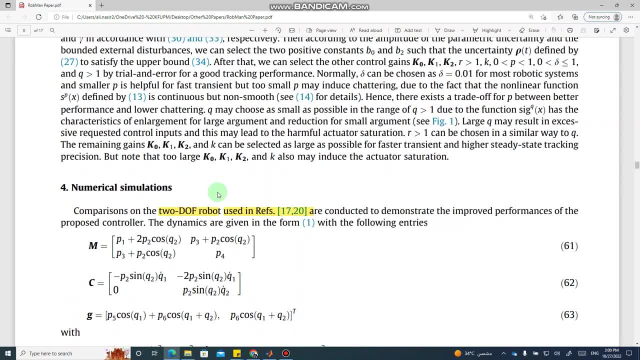 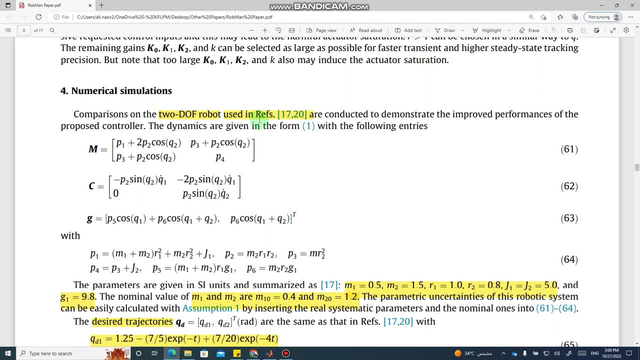 the control a little bit smoother. and this is the numerical example that we are going to simulate today here, this two degree of freedom robotic model, uh, robotic manipulator model, where m is. these equations, c, g, are given, where p1, p2, p3, p4, p5. 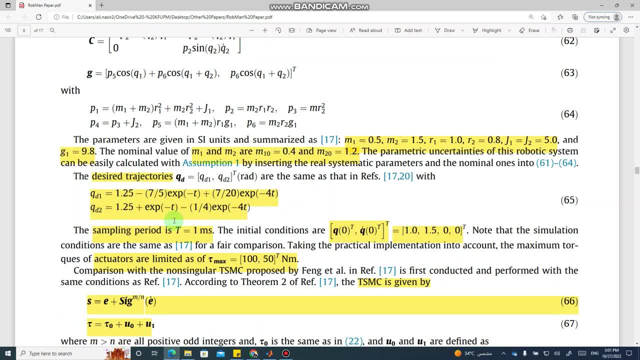 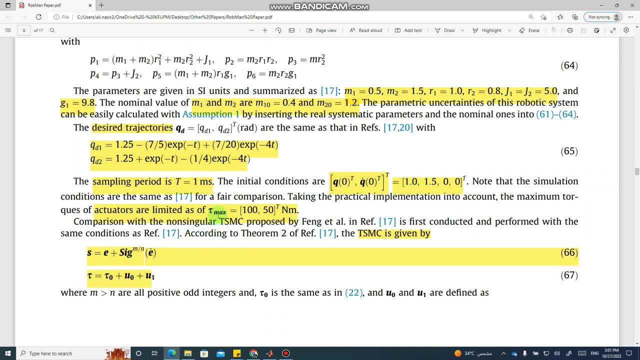 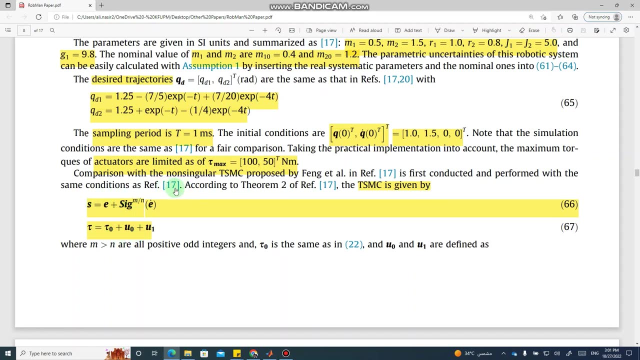 everything is given. these are the parameter values. they are also given. this is the desirable trajectory and the initial conditions. so everything is given. so they have compared their uh proposed controller with this controller which has been proposed earlier in the the one of the reference papers. i'm not going to simulate this controller, i am only interested in. 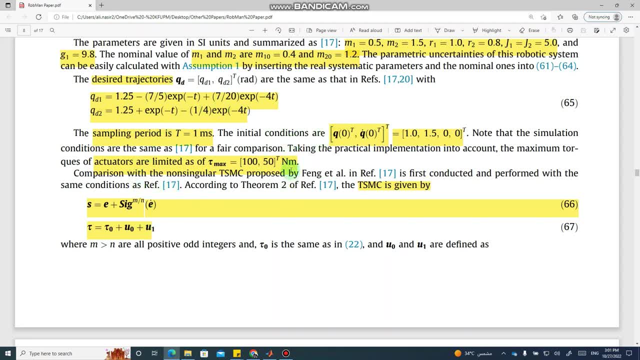 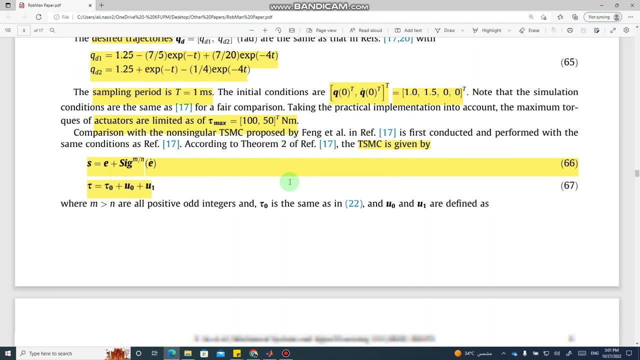 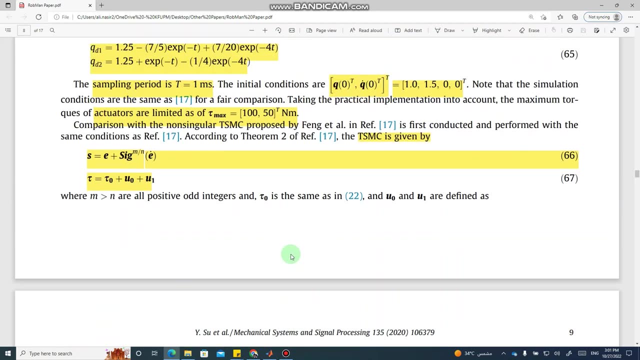 the controller that has been proposed in this paper. so we will be simulating only one controller that has been proposed in this paper and then later on you can go ahead and use this video to simulate more control laws which have been simulated in this paper, if you. 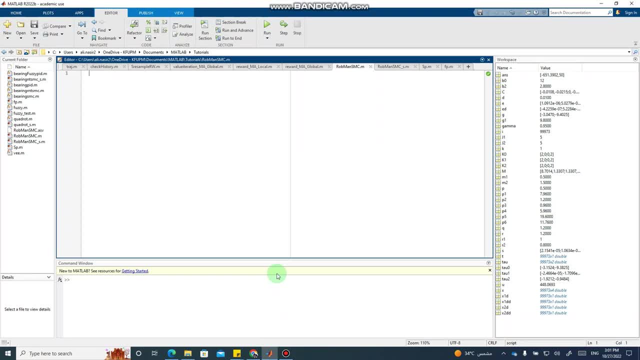 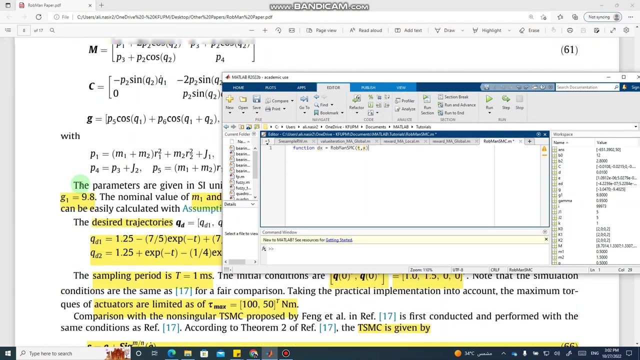 want to simulate more control laws, you can go ahead and use this video to simulate more control laws. so when we open the, when we open the matlab, we can just, you know, uh, write this, uh function. we can start writing the function file. first of all we have to write down the, the parameter values. so 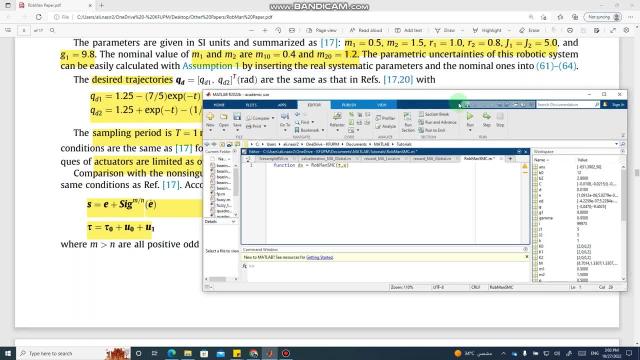 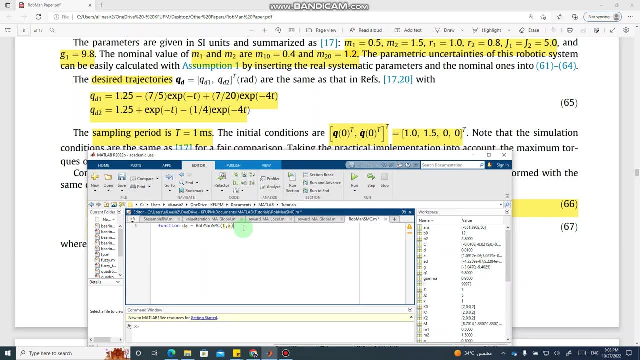 let me just scroll this up and you can see here. uh, let's put this down here so you can see here. these parameter values are given, so we can just write them down. so g1 is 9.8 m1 m2. these are also given r1, r2, the lengths of. 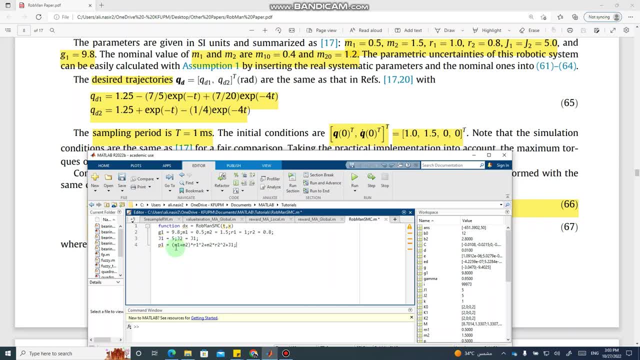 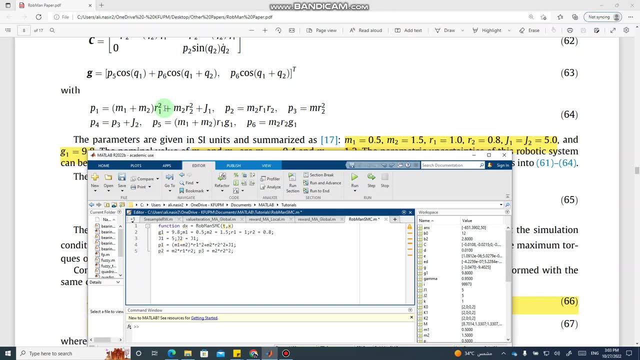 the manipulator. then inertia is also given: j1, j2, so p1, this equation, this is the this, this p1 equation, and then this p2 is also given here, p3, p4, here in p3, this is m r2 square, so i'm assuming this is m2 times r2 square, because that's. 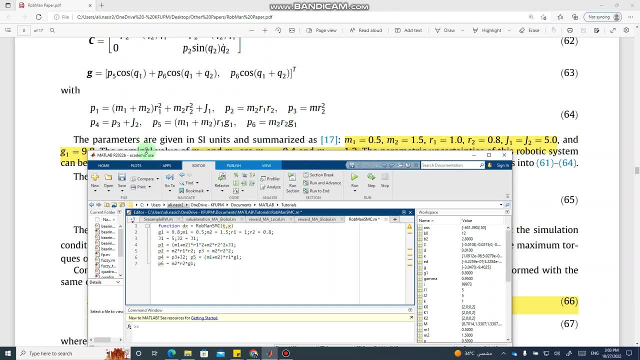 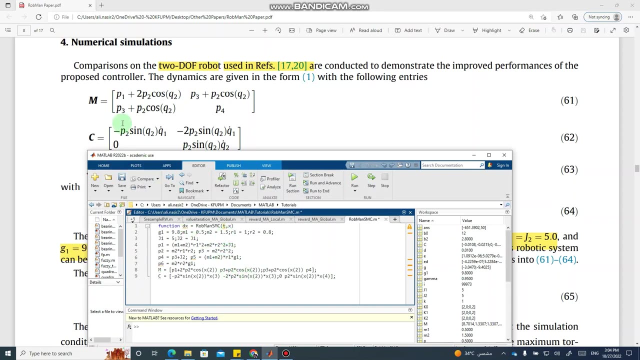 what only makes sense to me, then, p6 is this, this equation that we write here in the code, and then we write the m matrix, which is, which is this one, and then we write the c matrix, which is, which is this one: here, instead of q1, q2, we have x1, x2, and instead of q1 dot, we have x3. 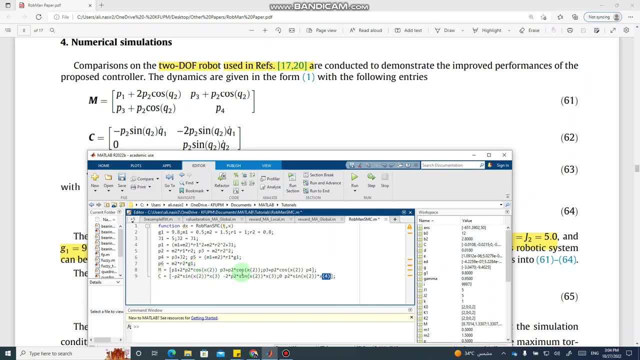 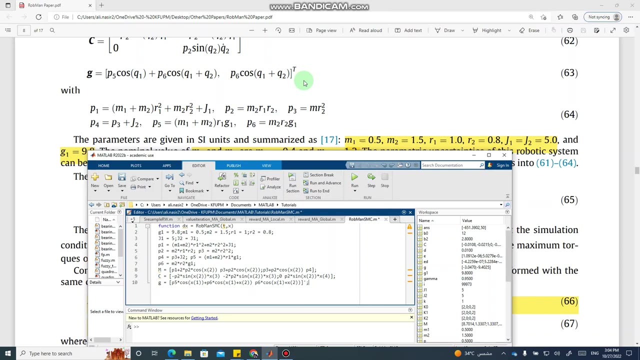 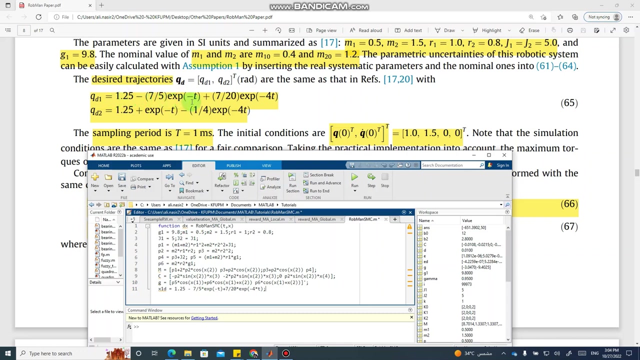 this is q1 dot and this is q2 dot, and this x1 will be q1 and x2 will be q2. so, having said that, we keep moving and we define the g- g is given right here- and then we define the desirable values of the trajectory: x1 desire, which is given here. x1 desire is q1 desire, which is 1.25. 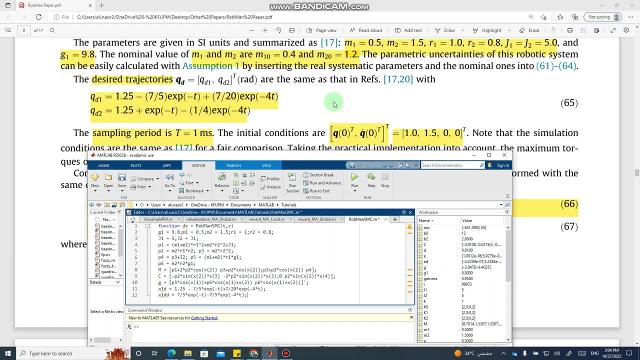 minus 7 by 5, exponent of minus t and so on. and then we define the derivative of x1, desire. you have to take the derivative manually. this is an exponential function, so very easy to take the derivative. we will be needing the derivative of the desirable state trajectory in the control. 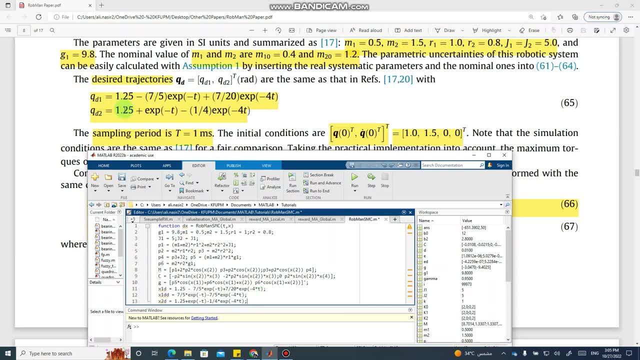 equation. so that's why we need it here. so x2 desire, this is q2 desire given here. so this is the same thing in the line number 13 of the code and then the derivative of x2 desire that we will be needing. this is the error. so error is x1 minus x1 desire, x2 minus x2 desire, so this is a. 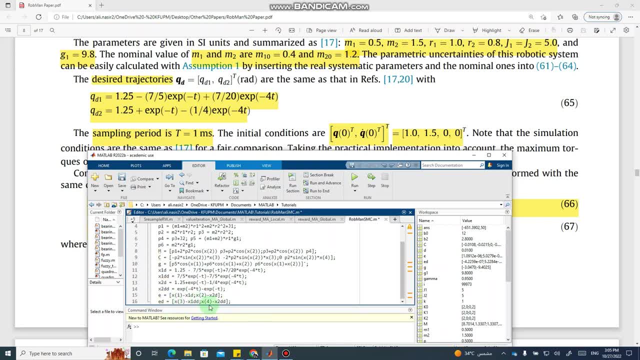 vector of 2 cross 1.. similarly, the derivative of error is x3 minus the derivative of x1- desire and x4 minus the derivative of x4- desire, so uh. derivative of x2- desire, so this. that's why we calculated these, these derivatives, because we will be uh, we need them in the expression for. 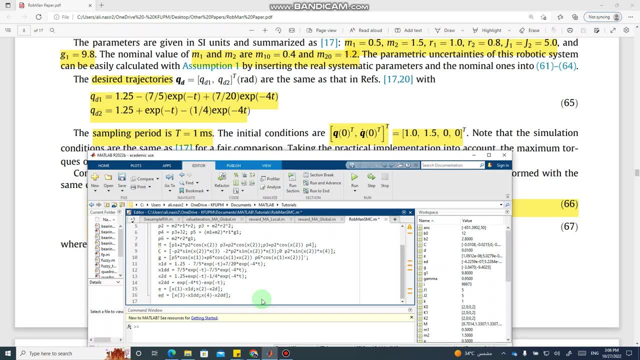 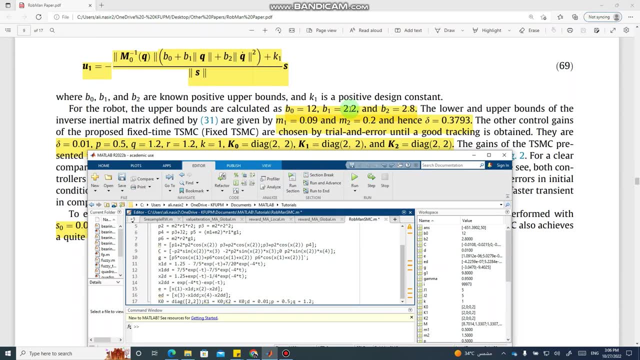 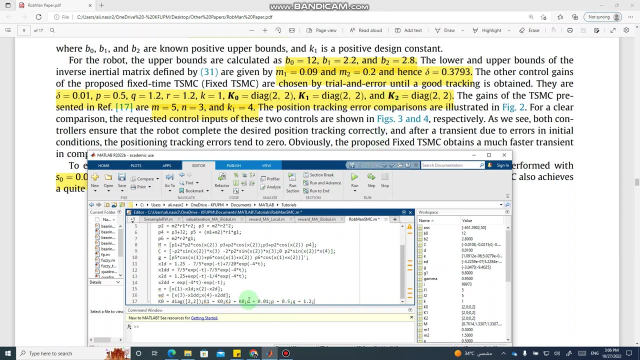 the derivative of the error. now we continue in this fashion. we define the, the parameters for the control, which are also given here. so k, naught, k1, k2, these are all diagonal matrix of 2 by 2. this is delta, p, q. these are also given in. 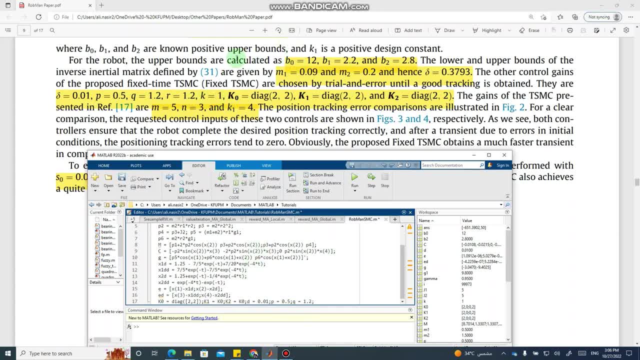 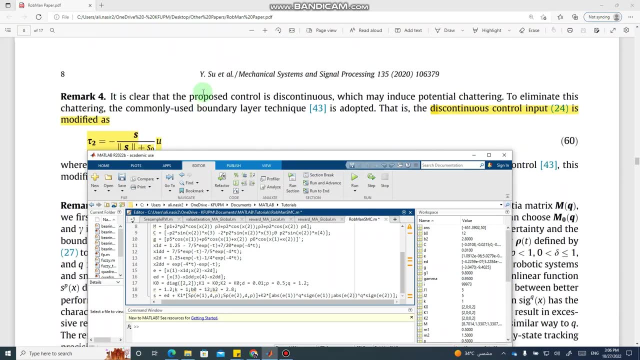 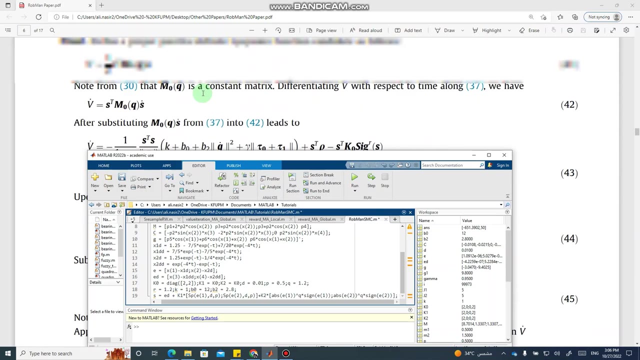 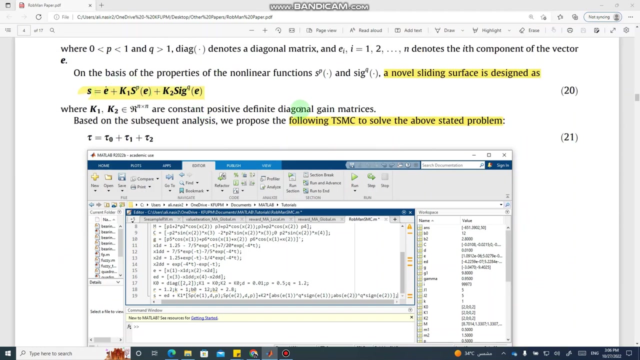 the paper: c, this is delta, this is p, this is q, r, k. so these are all values that are given in the paper. and then we continue writing this. now we go to this sliding surface, so we write the sliding surface which is given above: uh, here, um, you can say: this is: if you go up, yeah, here, so here, this is the sliding surface. 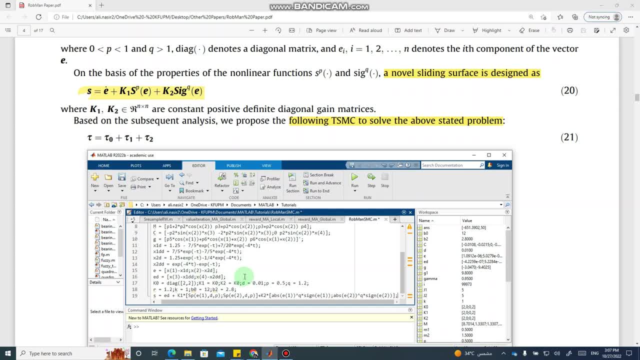 equation 20, which is line number 19 in the code, and then you can keep going. so within this line there is a sp function that we have used. so if you go, if you want to know what is sp function, let me show you. so sp is just this function, that if you need to define it like this, 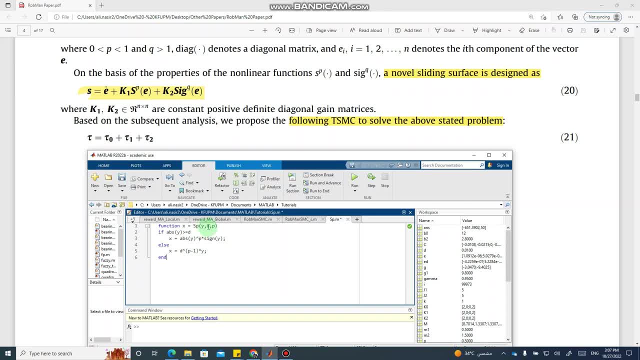 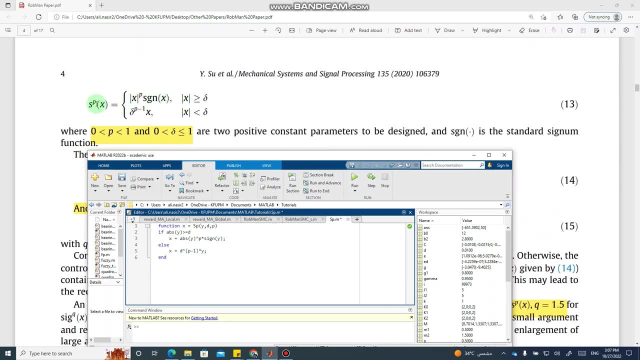 because in this function you will be needing the variable on which the function is called and you will be needing the value of delta and the value of p, because here sp is the defined in terms of x. but you don't need just x, you also need to know the delta and you also need 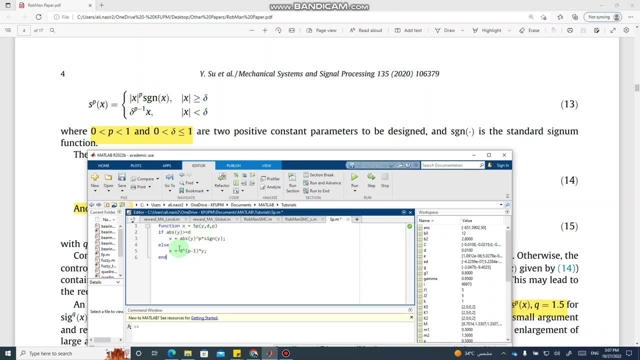 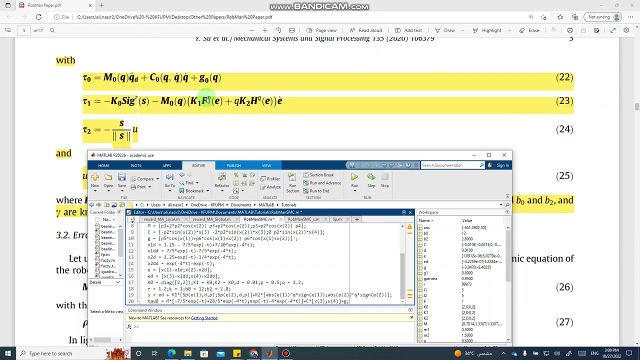 to know this p. so if you know, know this p and this delta, then you can apply this equation in the form of, if else in the function. so then let's save this, go back to this guy and continue writing our code. so tau 0, that is the function given here. 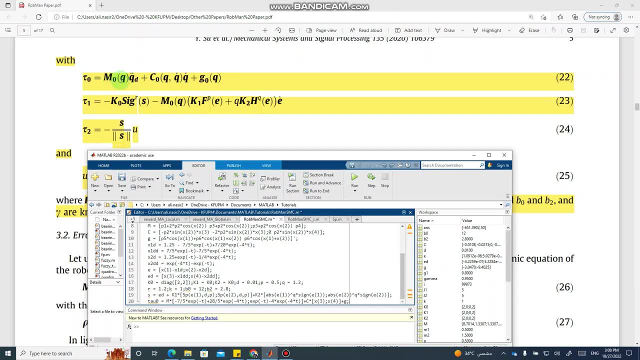 here. so tau 0, you just write it. so instead of using the nominal masses- although nominal masses are given in the paper, i have not used them because they are not very different from the actual mass- you can use instead of here: m, you can use m- naught, and instead of c, you can use c, naught. 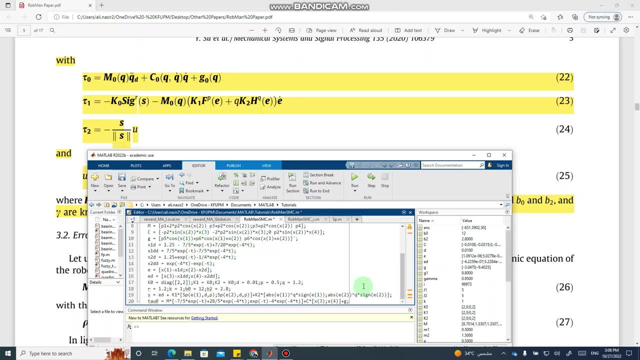 the only difference will be: the masses used in these two matrices will be the nominal masses instead of the, the actual masses. so that's then. next is the. this tau 1 equation, which is this one: here you have sig power r s, so i have not defined a separate function for this. i 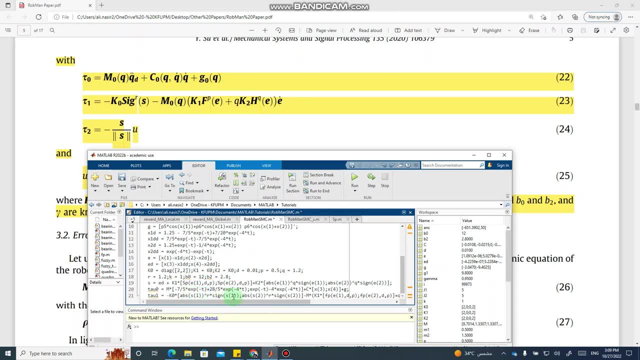 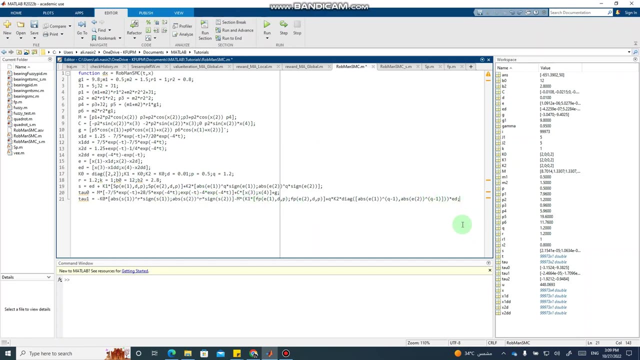 have just used absolute of s1, time absolute of s1 raised power r into sine of s1. so this is sig power r of s1 and similarly sig power r of s2. so this is. i just maximize this so that you can see here this is tau tau 1 equation and then gamma. it's not explicitly given in the paper but i know. 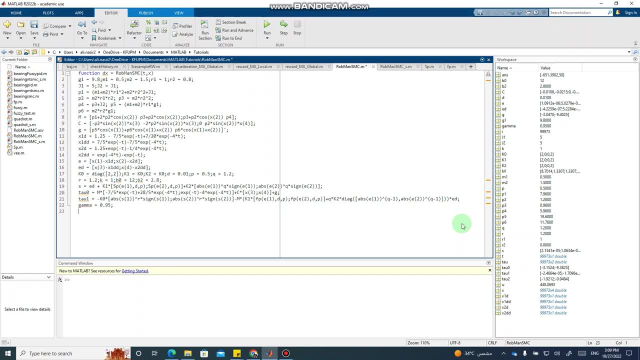 that gamma is some value between 0 and 1, so i can just choose a value to be close to 1 to be on the safe side. u is given in the paper. you can see here that 1, 0, 1 is internal value of sigma and sigma's Rodrigo state gigabit. um going to peak is greater than 1 diameter and 6.06 times 0, 3 where you put the sigma, Almost von Hanfield's distribution × delta, naught power, fa, por-1, s, 1 and similarly sig power r of s2. so this is- i just maximize this so that you can see here this is tau, tau, one equation and then gamma. it's not explicitly given in the paper but i know that gamma is fixing the table here and 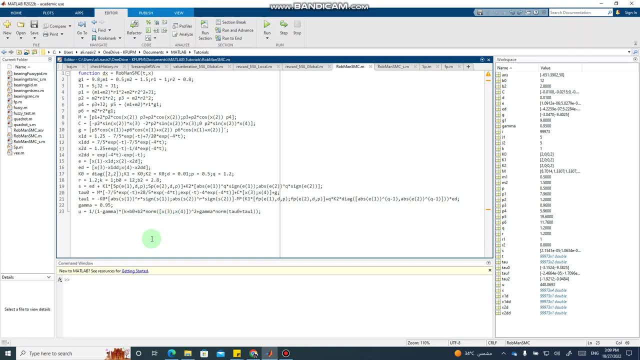 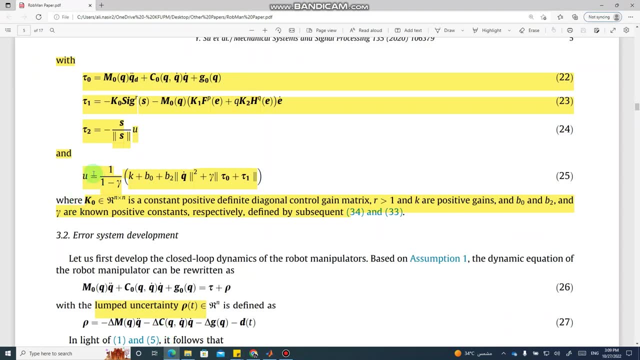 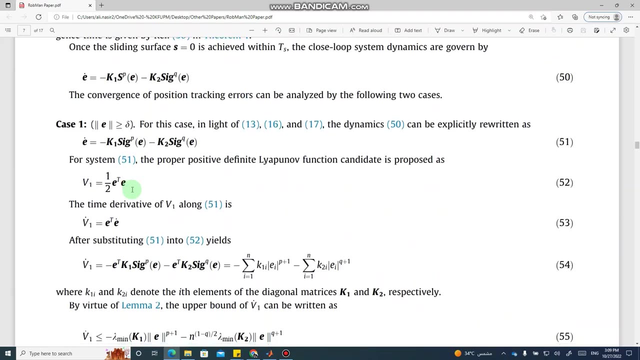 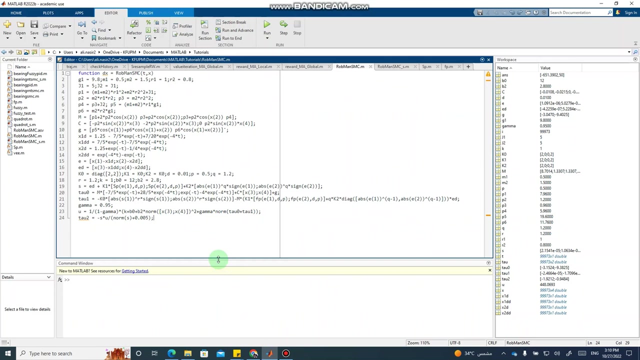 that u is this equation. so writing this equation in the, in the code right here, and then tau 2 is also given in the paper. but i have not used this tau 2 like this one. i've used the tau 2 which is given below this, this one. so this tau 2 is better, so i've used this one, and then tau is just tau 0. 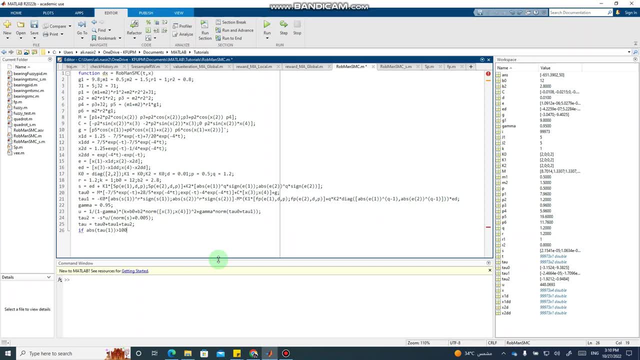 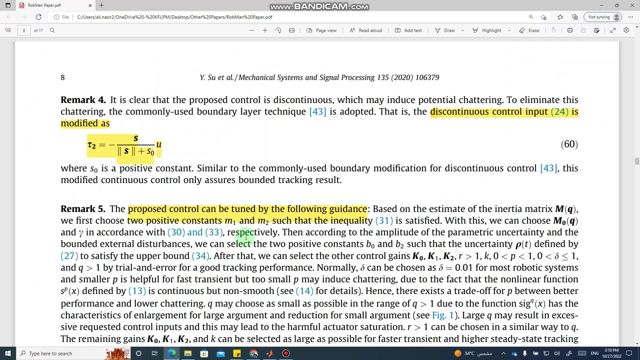 plus tau 1 plus tau 2. and then there is some restriction on the control signals. so in order to reflect the actuator saturation, they have put restriction on the control signal that one of the control signal cannot be greater than 100 and another one cannot be greater than 50. so this we can apply here. so in the paper i think this is. 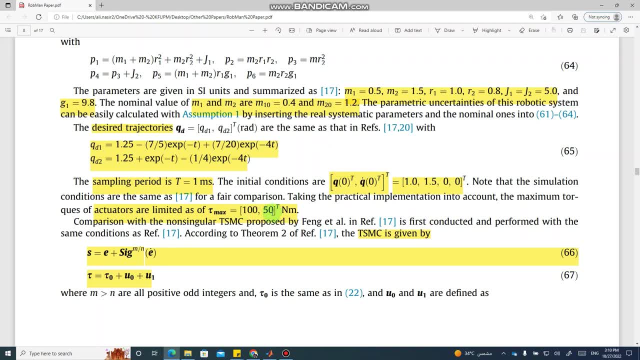 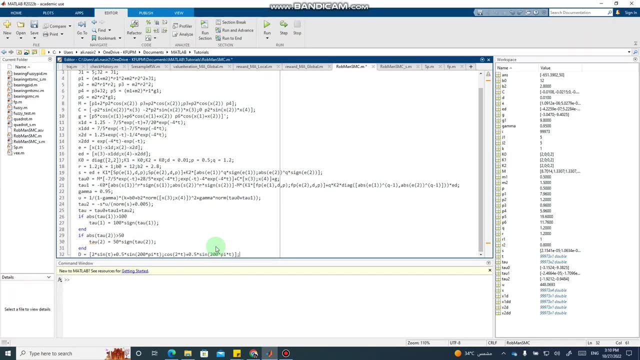 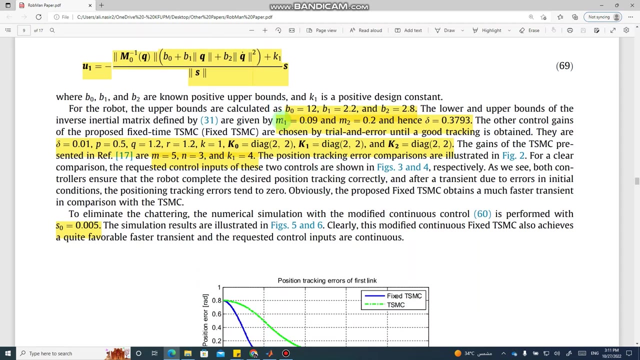 written somewhere here. so tau max is 100 comma 50. so one control cannot be greater than 100 and another cannot be greater than the second. one cannot be greater than 50. so next we write this: this d part, the disturbance in the system. that is also given. let's see, it's given. so these 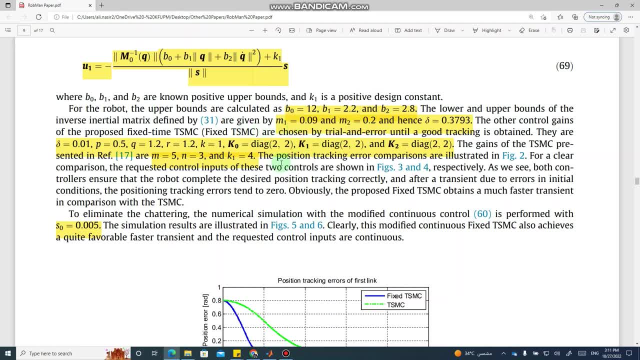 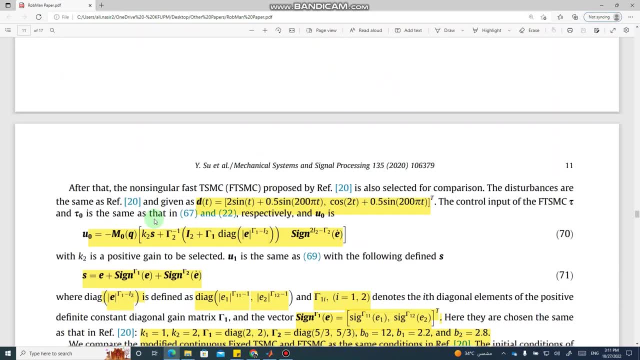 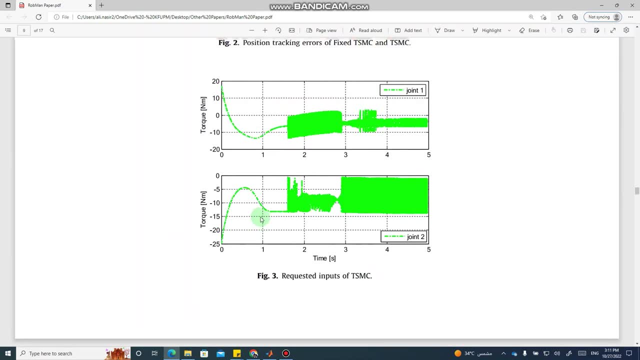 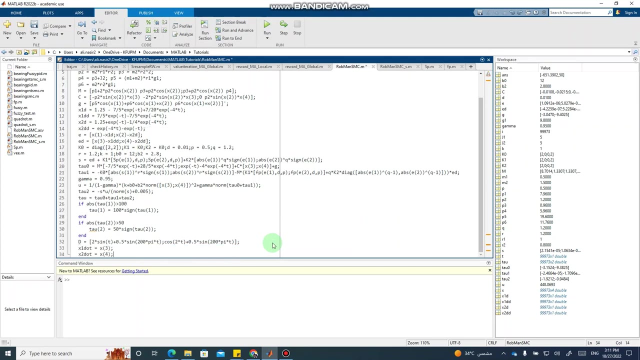 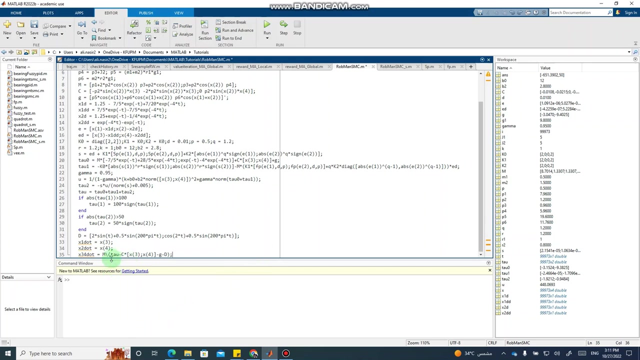 are the. these are, these are the m1, m2 masses and they have also given nominal masses somewhere around here. but anyways, so this disturbance is this guy, so this disturbance i have used here, and then you can write the dynamics, so x 1 dot equal x 3, x 2 dot equal x 4, and x 3 and x 4 dot. i have combined. 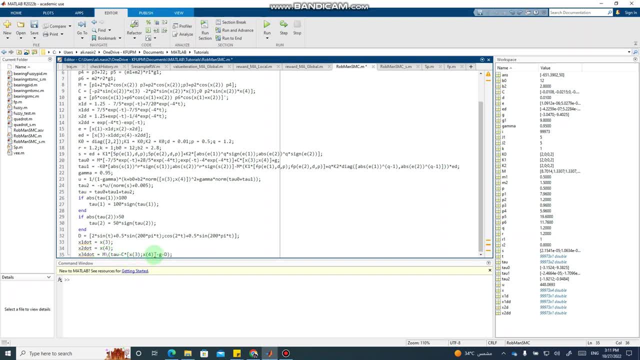 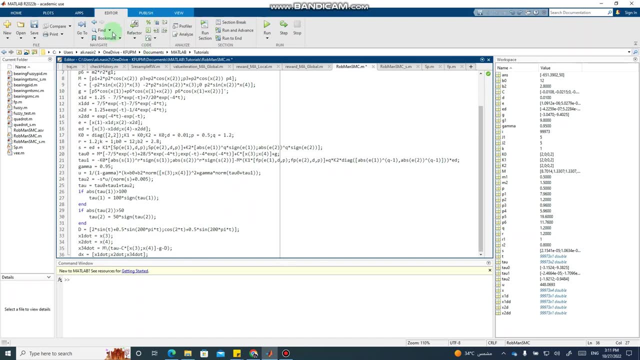 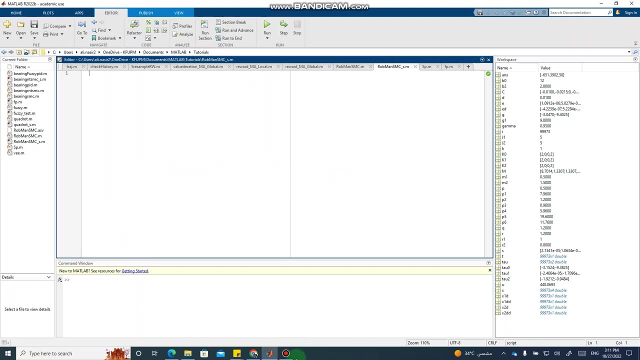 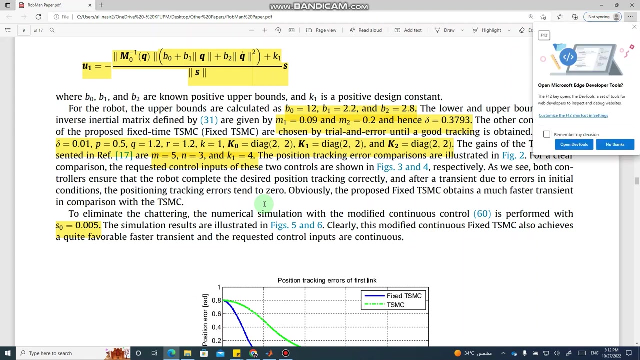 them into a single equation. this is m inverse tau minus c, psi c times q dot minus g, minus disturbance, and then this completes our function file, so we just save it, and then next we go into the robot the script file for for this simulation. all right, so 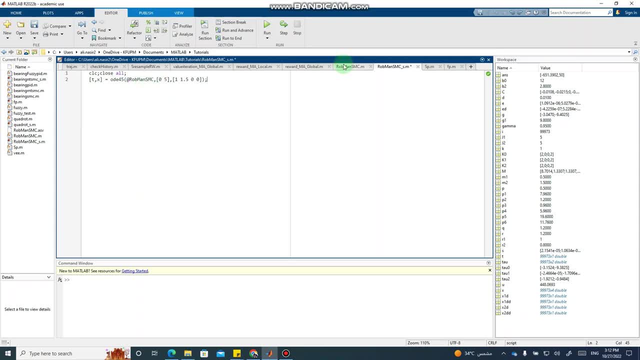 for the script file. we just use clc, close all. we call the ode45 function and we call this this function. uh, rob, rob, manipulator, smc, that we just completed. and then we have these. okay, these parameter values are repeated because i'm going to, i'm going to show you the plot of the control signal as well. so, in order to so, this code is: 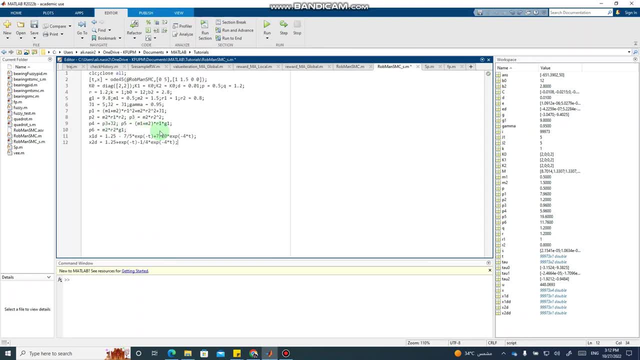 basically the repetition of this code that we written here. so we need this repetition because we want to plot the control signal. so x1 desire, x2 desire- notice that the t here is no longer just a scalar time, it's a vector that will be computed from ode 45, so it will be a lot of values and then tau. this is the initialization. 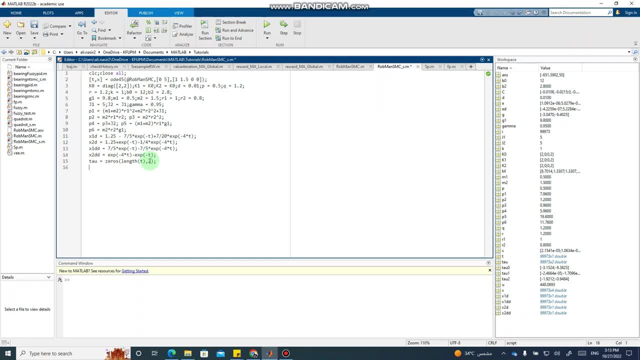 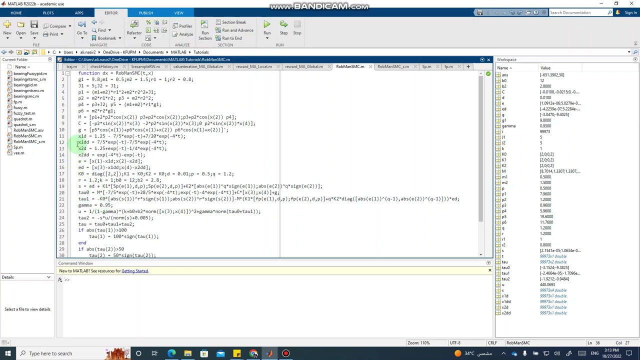 of the control and the control values will be as much as the number of values in the time signal and it will have two- call two columns because we have two motors in the system. so now we have for loop for one. to length of time we recursively define all of the remaining things inside the for loop because we need controller. 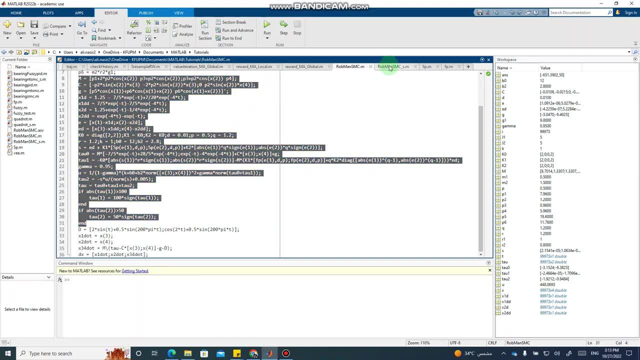 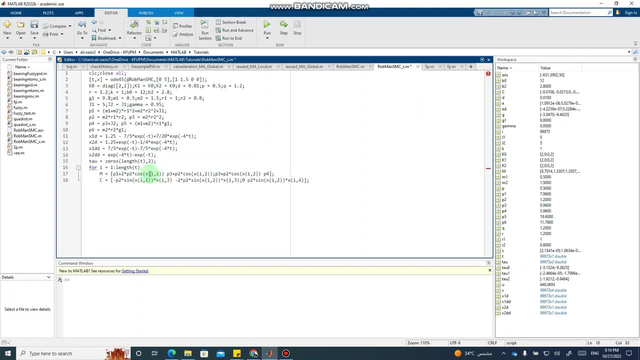 at every time step. so the code from here to the all the way down here, so this code will be copied in in here. so the only difference is, instead of using x2, you will use x of i comma 2, instead of using x 3 or x 1. so wherever there is a x vector, there will be, you will be using x i comma 1, x i comma 2. 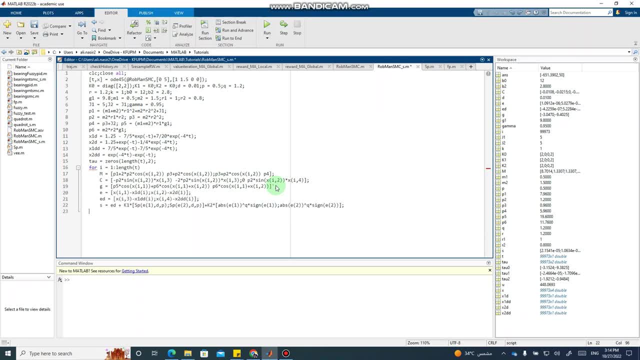 x i comma 3 and x i comma 4. so this will be the only difference, and then you can just recreate the same code sliding surface: tau 0, tau 1- you, and whenever there is, also wherever there is t. so instead of t you will be using t of i, because t and x have been computed here so they 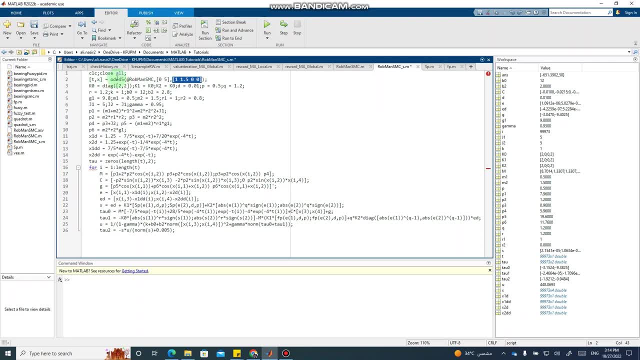 are no longer like single values. so these are the initial conditions that are given in the paper that we provide to the ode 45 function, and we simulate for five seconds, because in the original paper results have been simulated for five seconds. we can also simulate for longer if 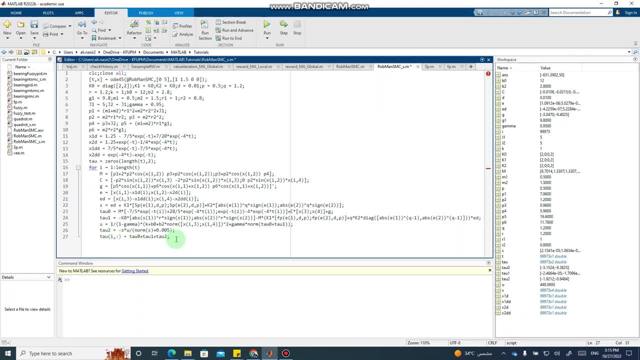 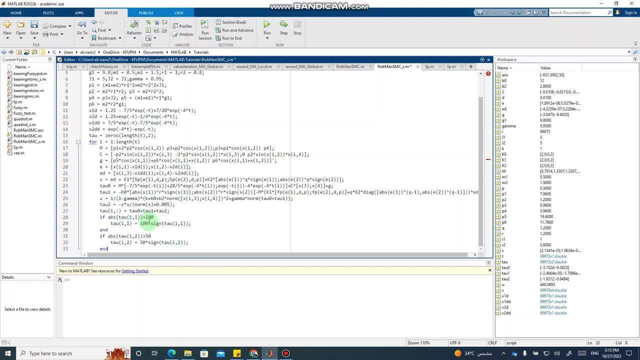 if you want, then, uh, this is the tau i. so, uh, ith control effort, you will calculate from tau 0 plus tau 1 plus tau 2, as you do in the other file and as has been done in the paper. so this is the restriction on the control, that one control signal cannot be greater than 100 and another. 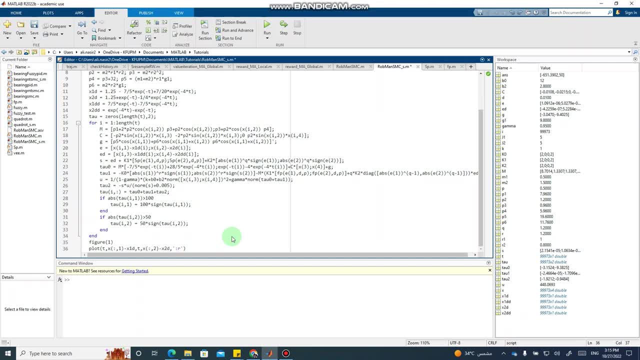 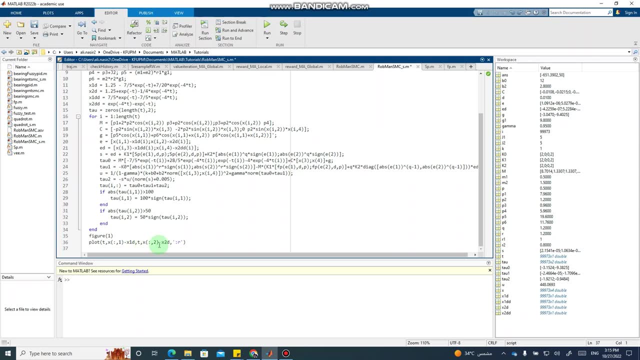 cannot be greater than 50.. now, now you can plot this plot: x1, x2, x1 minus x1 desire, which will be the error in the first joint reference tracking, and x2 minus x2 desire, this will be the error in the tracking of the second joint. then this will be the plot of the controllers. so 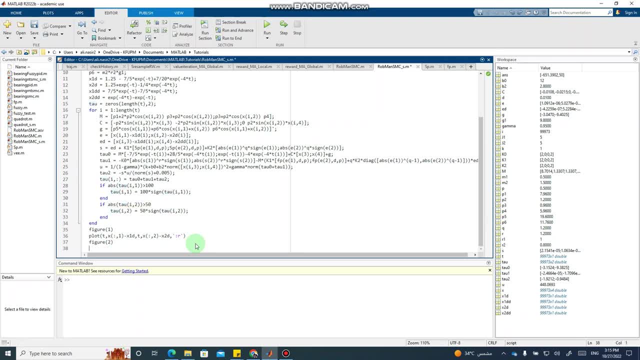 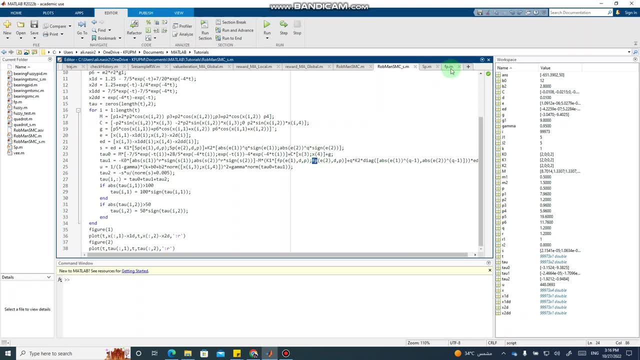 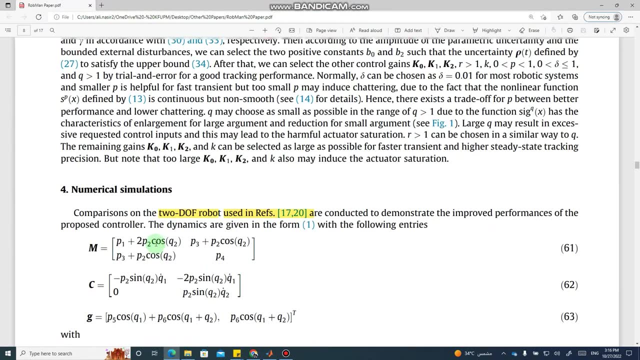 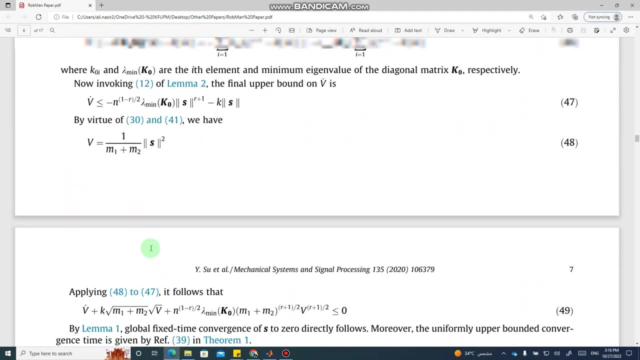 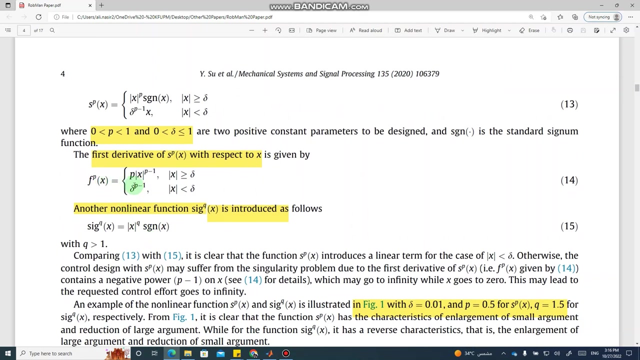 so this is where we are, so we just save it and notice this. we have also used another function, fp, here, so fp will be the function based on on this file. so here this: there is this function fp. so there, this, this function fp. you can write this. so in order to do fp, you need to know x. 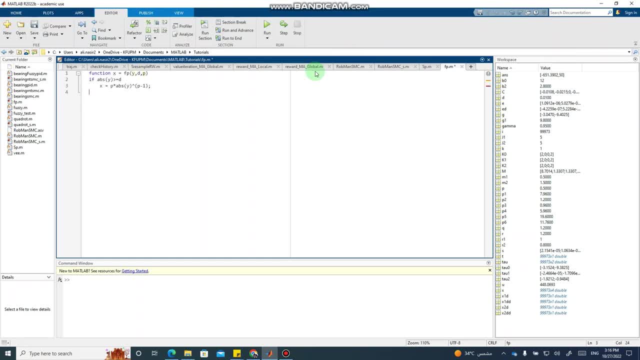 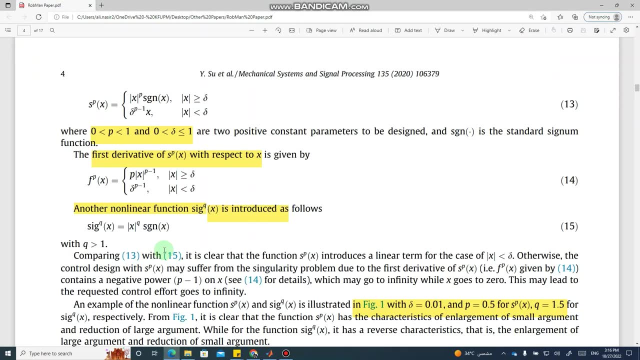 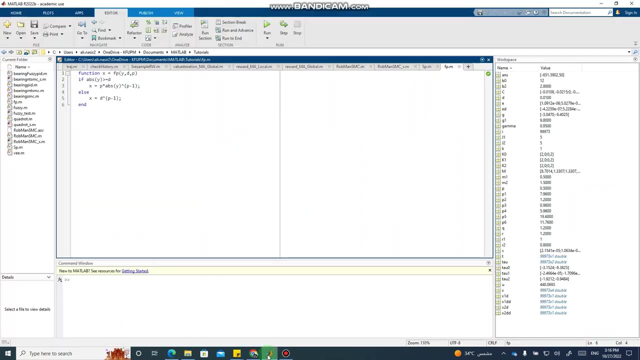 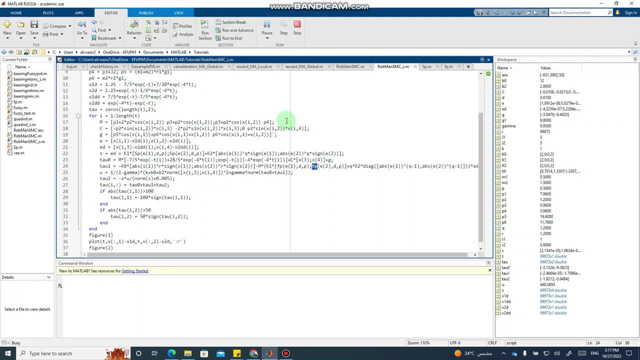 you need to know p, you need to know delta, so this fp will have three inputs and then you can just use, if else, to implement, implement this, this, this conditional definition of the function. so then, finally, when you have done everything, you can just go back to your script file and you can run this file.